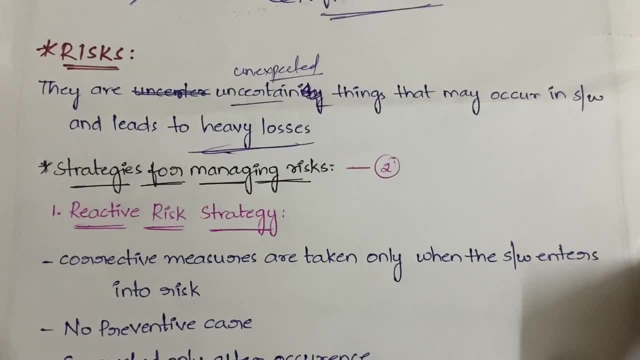 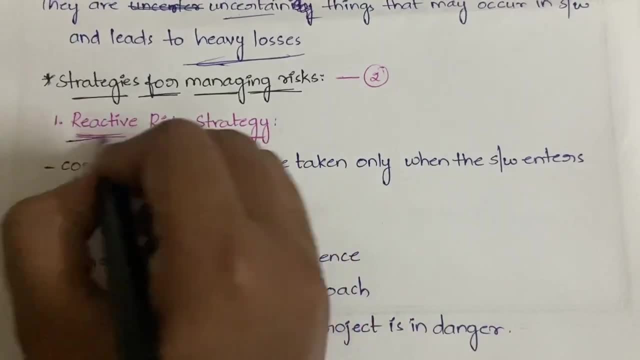 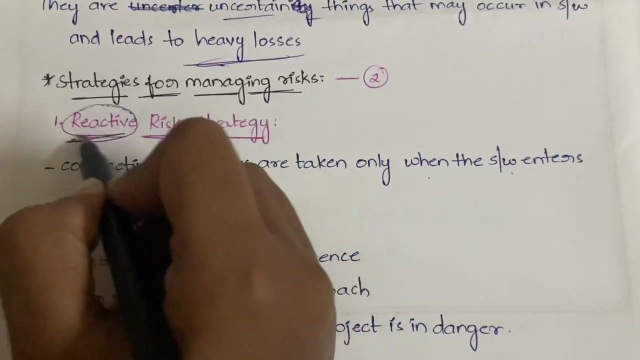 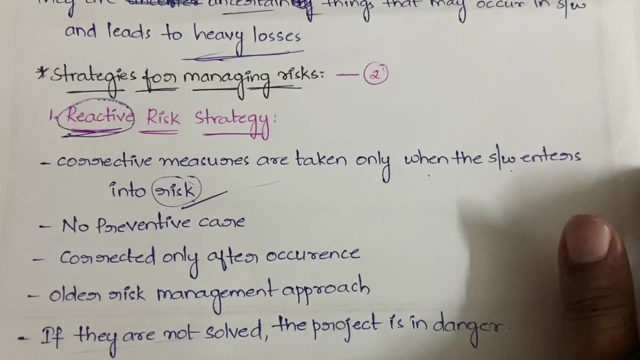 Differences between them. now, Got it? So first, you're clear with the definition of the risk. right Now let us see what do you mean by the reactive risk strategy. So first of all, reactive: it says that the corrective measures are taken only when the software enters into the risk. That is, we will react only when the software is entering into the risk. Got it? So? when previously we will not take any preventive measures for the risk. 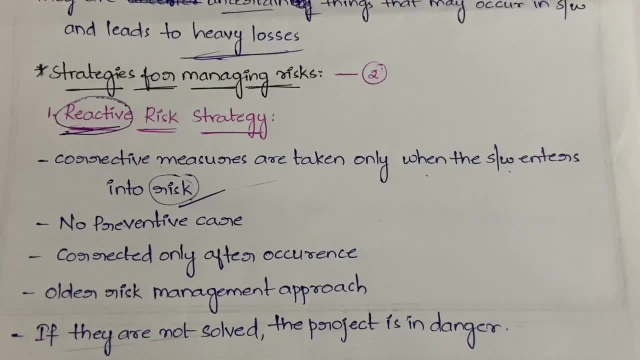 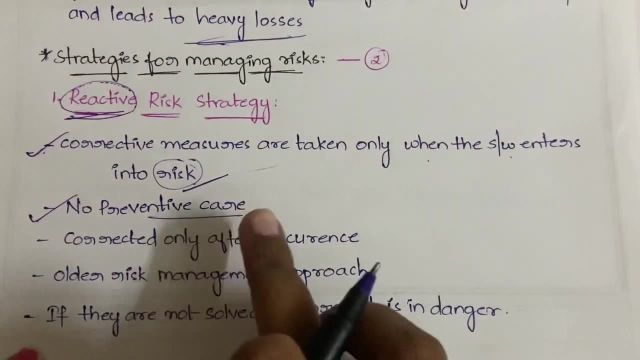 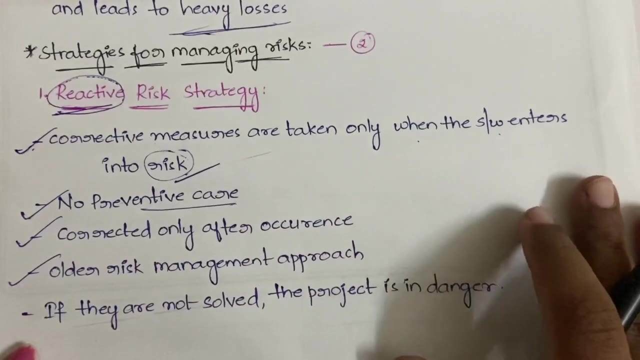 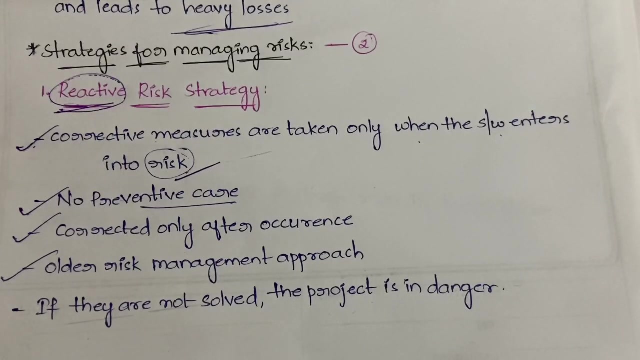 After it enters into the risk, then we will realize, then we will react, then we will wake up, Okay, simple. Next, no preventive care is taken. That is what I said, And correcting or corrected only after occurrence, That is, only after it occurs, only it is corrected. Older risk management approach. Of course it is older because nowadays everything is being advanced right Initially. only we are predicting everything. So that is why it is a older risk management approach. And if the risks are not solved, the product is obviously in danger, Because we have already 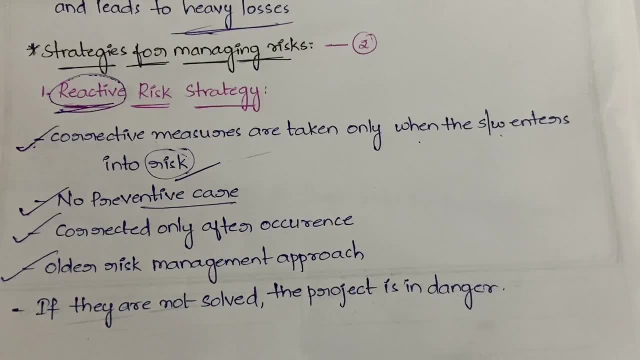 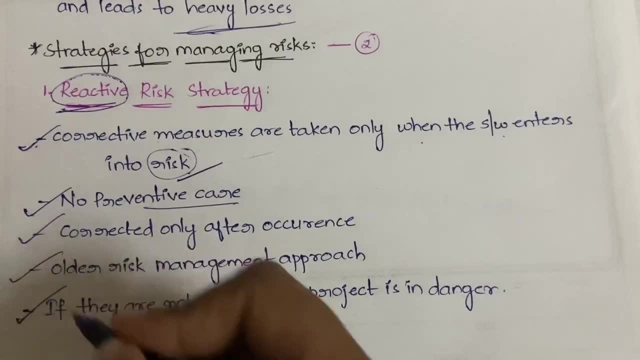 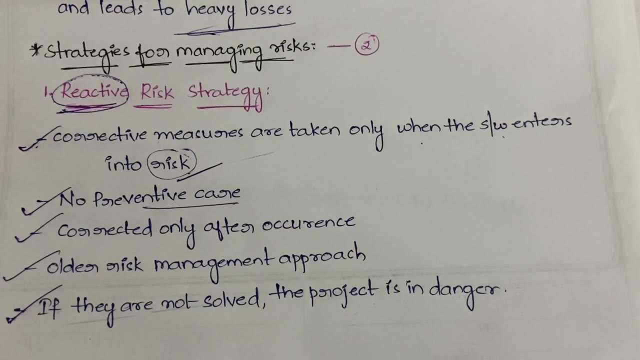 you know already, risk has occurred. So if that risk is not removed, because of that risk, so many risks may come right. So that is why, if it is, if they are not solved within time, then the project will be in the danger, Got it? So this is reactive risk strategy, which means we will react only after the risk occurs. Got it Previously. we will not take any preventive measures. Now let us see: what do you mean by proactive risk strategy? Second one is proactive risk strategy. Here it is completely 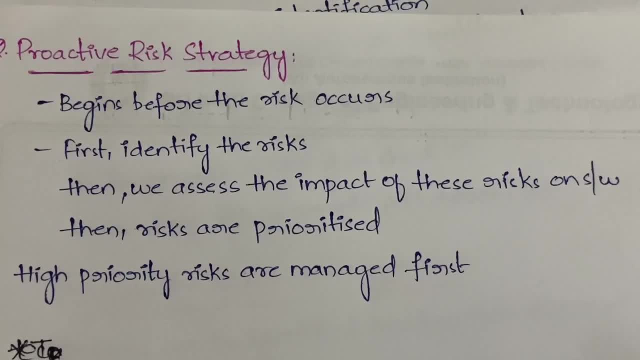 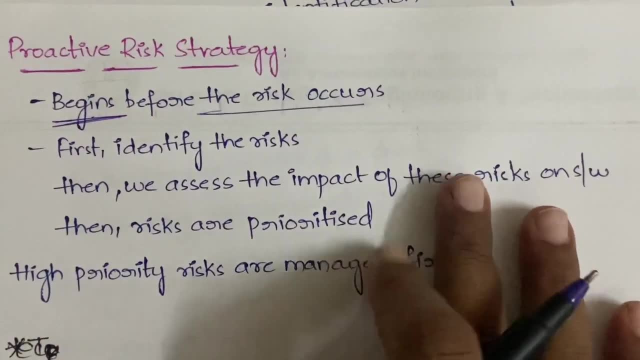 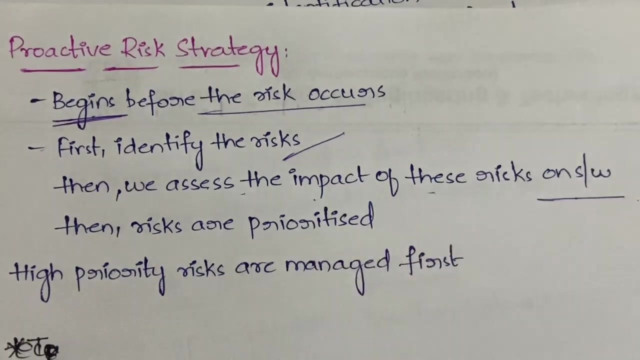 opposite to reactive risk. In reactive, what we do once the risk is occurred, then we start right here. It is not like that. It is big. it begins before the risk occurs. Got it. First it will identify the risk. Next we will assess the impact of these risks on the software. That is, how much impact it is going to create on the software, whether it is critical or medium or moderate or high, or the project is completely going to crash or it is not going to affect like that. First it will assess the impact of that. 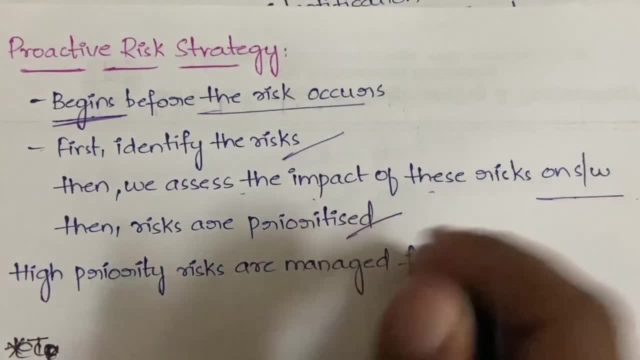 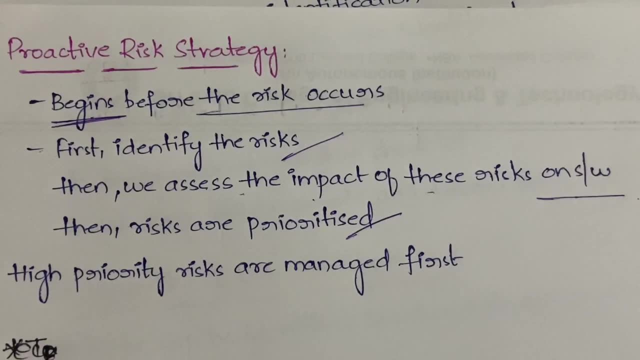 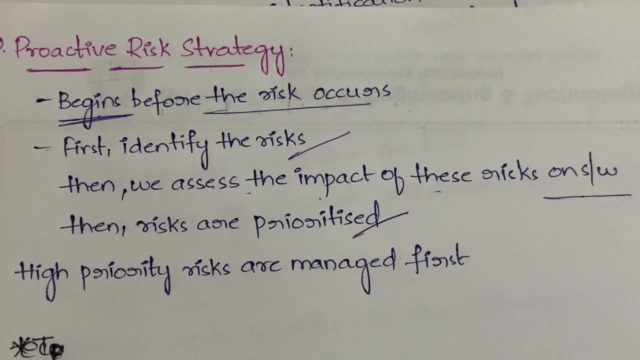 risk on the software. next, the risks are priorities, that is, you will be prioritizing the risk based on their impact, that is, which is having more impact, that has to be solved first, right? so like that, yeah, high priority risks are managed first, high priority risks will be solved first, then you will. 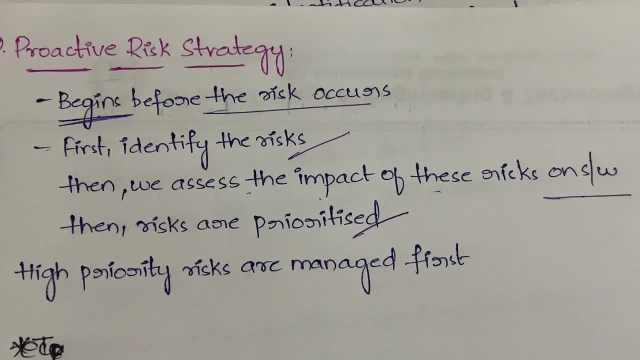 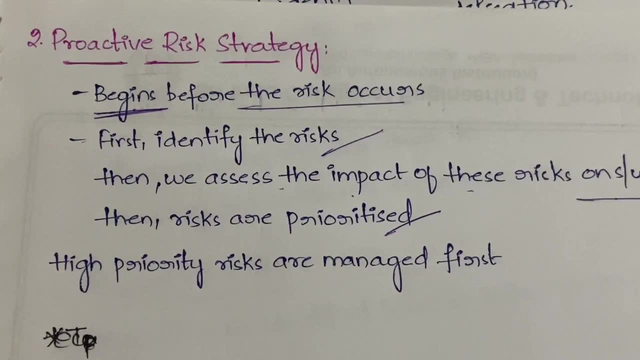 be going to the more priority ones. right got it. so this is the proactive risk strategy. proactive, reactive. the only difference is: reactive, you will react only after it has occurred. proactive, that is before itself, before the occurrence of the risk itself. you will be very active, you will be taking 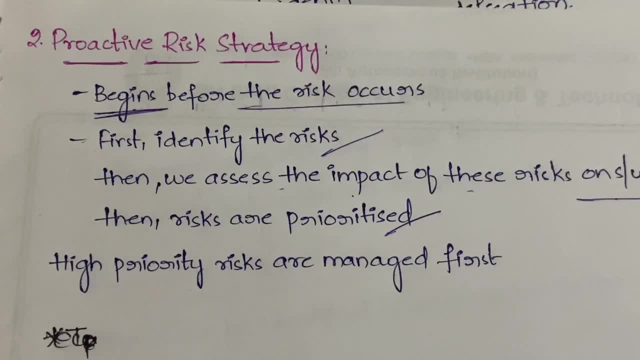 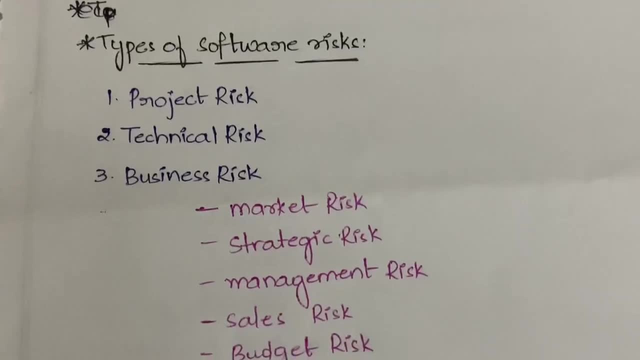 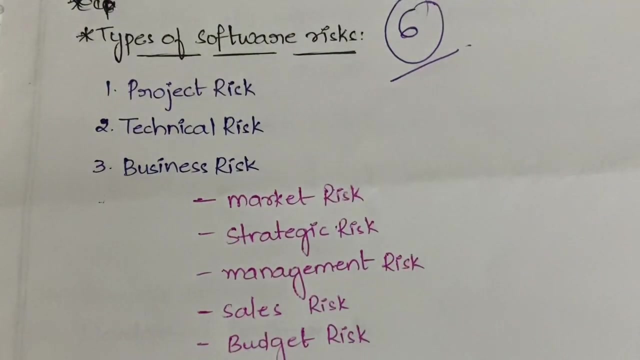 preventive measures and you will be identifying the risk, prioritizing them and solving them based on the priority basis. got it now next. so now we are going to see what are the types of software risks we have. okay, we actually have six types in total. six types of software risks. 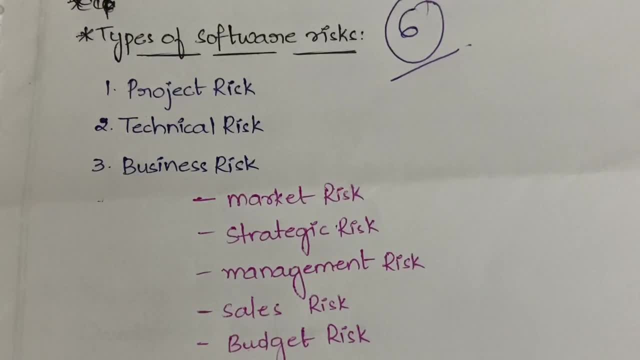 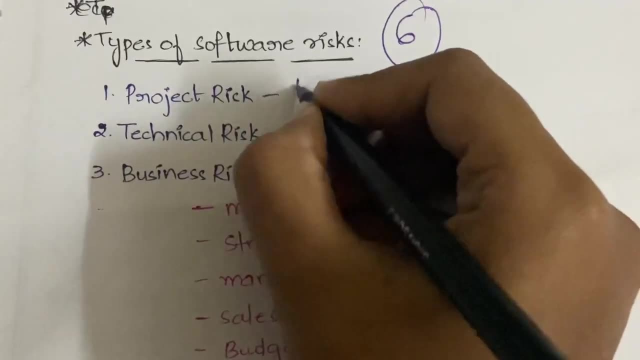 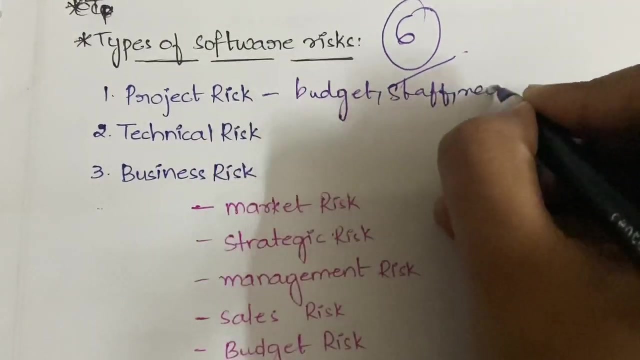 we have. so let us see in detail. so the first one is project risk. so what do you mean by project risks? what comes under project risks is nothing but the risks in budget, budget and staff requirements, schedules. so all these will come under the project risks. okay, the risks which are associated with. 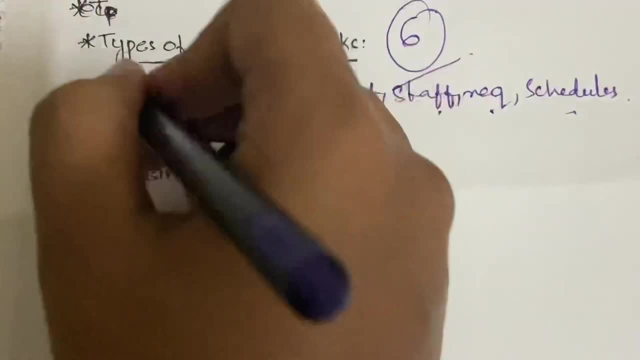 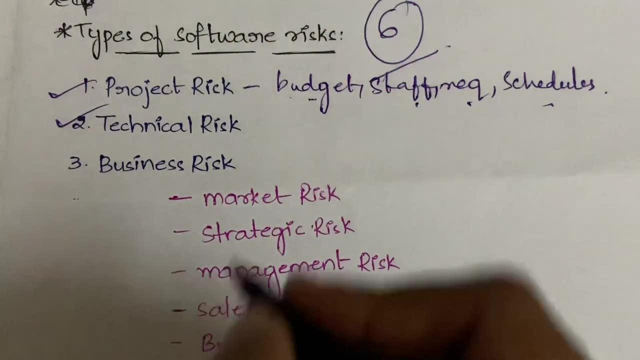 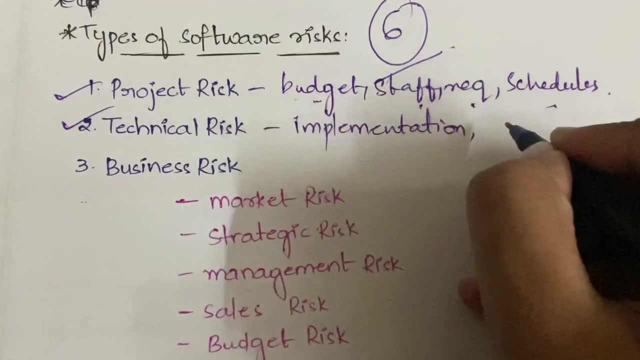 budget or staff or requirements or schedules. all these will come under project risk. next comes the technical risk. in technical risk, you will have some implementation risks, like when you are designing which you have thought so during implementation you will be getting the some risks. and while implementing the interfaces also, because this product will have several 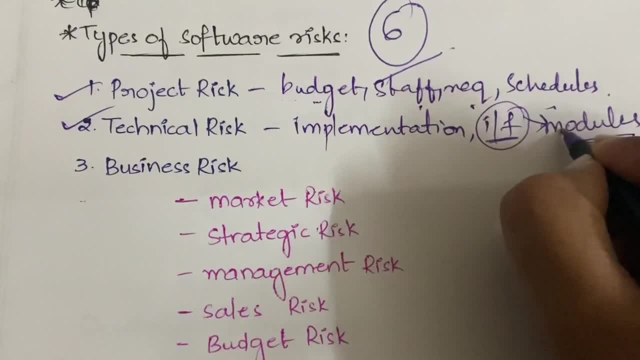 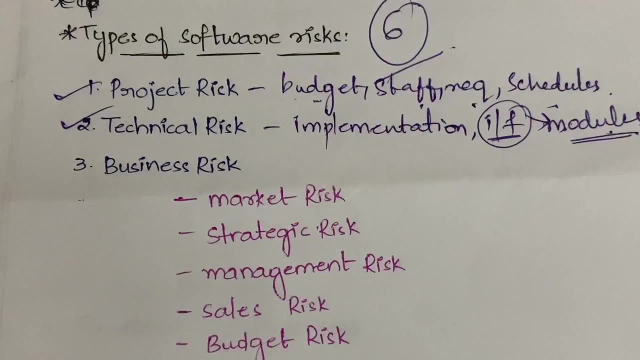 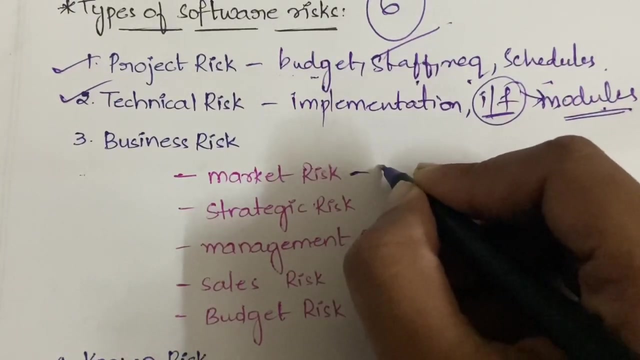 modules, right. so among all these modules you need to establish interfaces. so while establishing interfaces also you may get some technical risks. next comes the business risk. so again in business risk we have some subtypes. okay, first one is market risk. market risk is nothing but the risks which are associated with market, like no customers in the market to buy our product, like that. 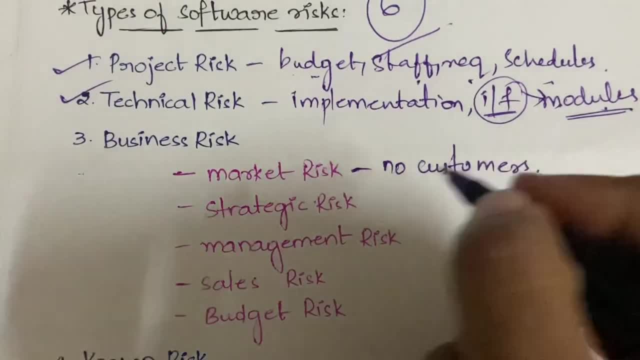 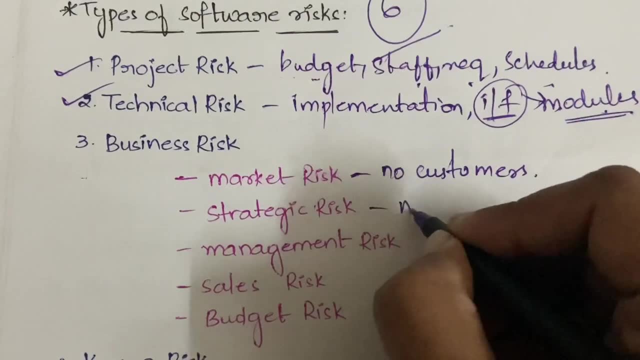 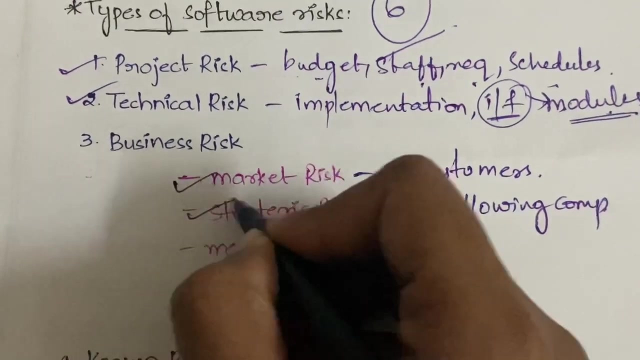 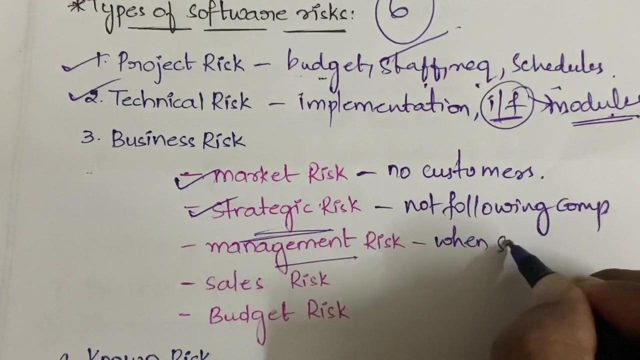 no customers. and next comes the strategic. strategic risk is nothing, but if the product is not following the company policies, then the strategic risk may not following. not following company's policies, then strategic risk will arise. okay, next comes in management risk. management risk is nothing, but when senior manager leaves, like i'm telling you the example: when senior manager leaves. 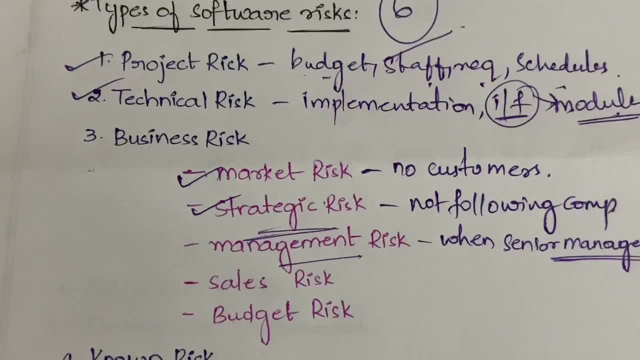 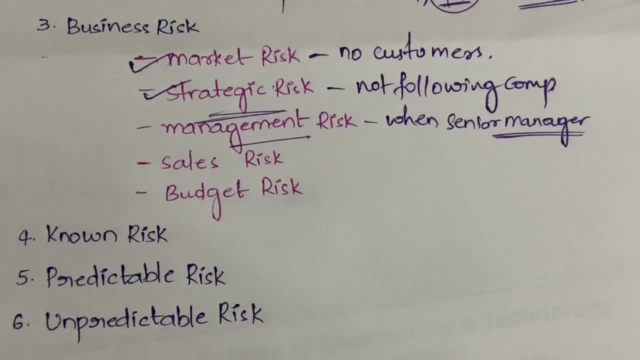 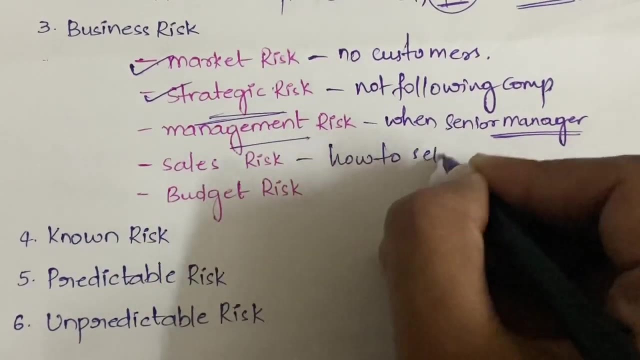 new organization because he knows everything, um, he is completely habituated to the organization and all right. if somebody new person comes, then everything has to be again freshly taught to that person like that. next comes the sales risk. sales risk in the sense we are not clear about how to sell. it's not not having customers. not having customers will. 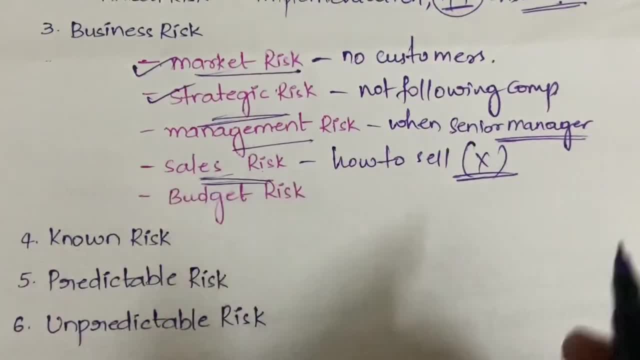 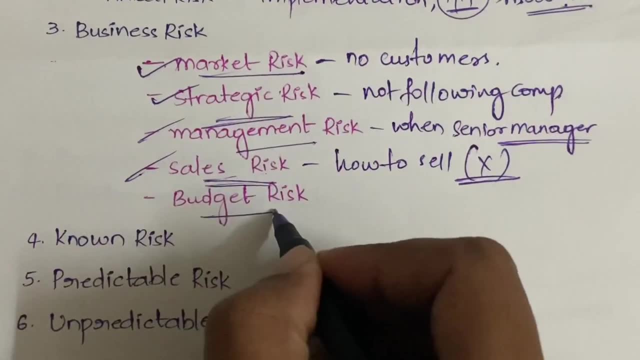 come under market risk. so when we don't know how to sell, when we don't know how to sales, how to make sales and we don't know how to advertise the products, and all you will be getting the sales risk risk. next comes a budget risk. budget risk is nothing but loss in budget or low budget. 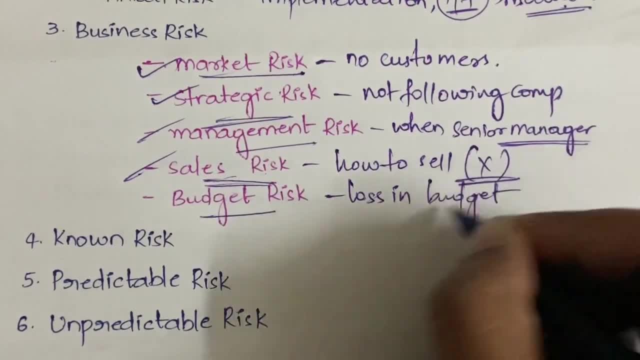 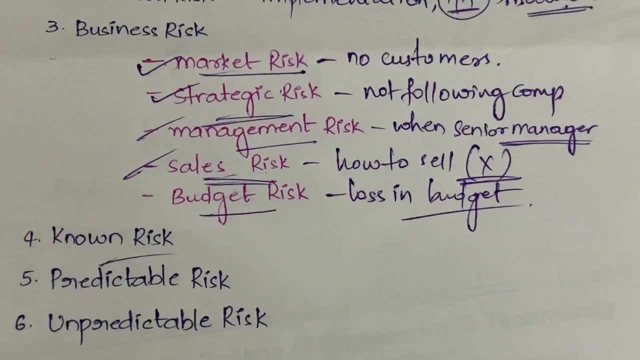 like that. okay, so these are the businesses- different types of business risks you have. next comes a known risk. known risks are nothing but which you already know. okay, this will definitely happen. uh, whatever we do, how much, ever, perfectly we do or not, this will definitely happen. so we. 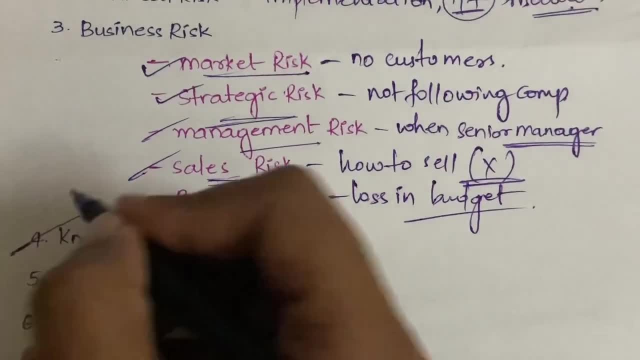 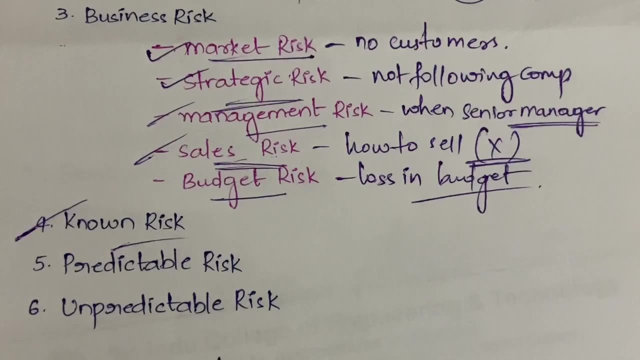 have to somehow prepare to clear this. that is what known risk means. next comes a predictable risk. predictable risk is nothing, but you can predict. see when we are, when you are implementing or when you are doing the interfaces, then you will get right. so okay, maybe this may happen, maybe this. 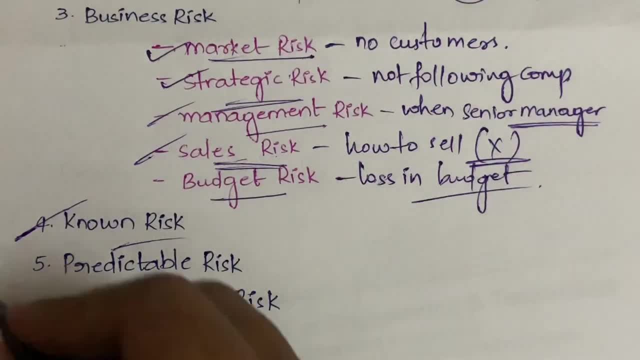 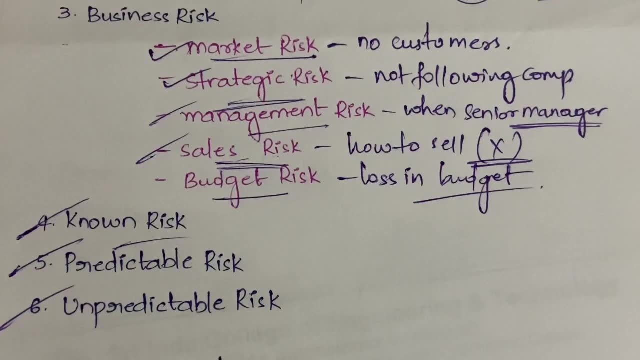 risk may occur. so you'll be just predicting the things, that's all okay. unpredictable risk in the sense you cannot predict that you can, you will not even think of that area. risk may happen in that area, you will not even think in that way. okay, that is what. unpredictable risk which you don't predict. 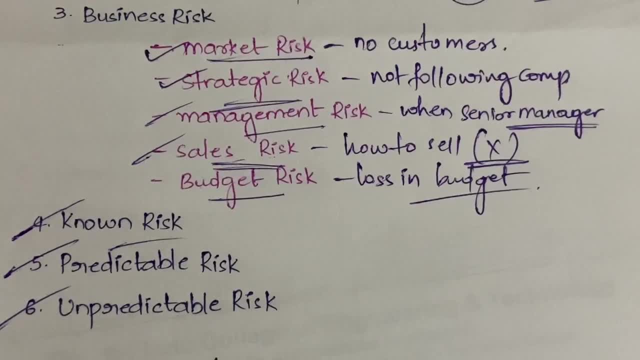 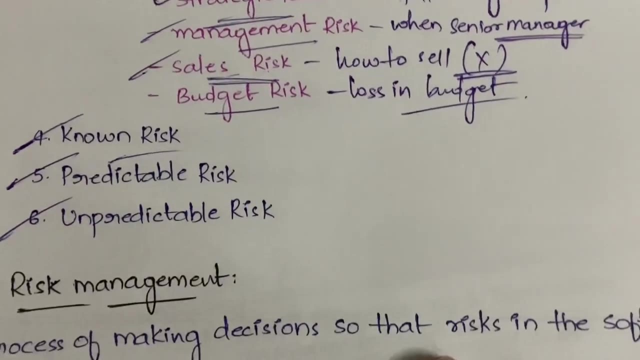 which you cannot even imagine or expect. okay, this is about the types of software risk. we have total of six types: project risk, technical risk, business risk and again business. we have subcategories, known risk, predictable and unpredictable risks. got it next. so the next definition that we are 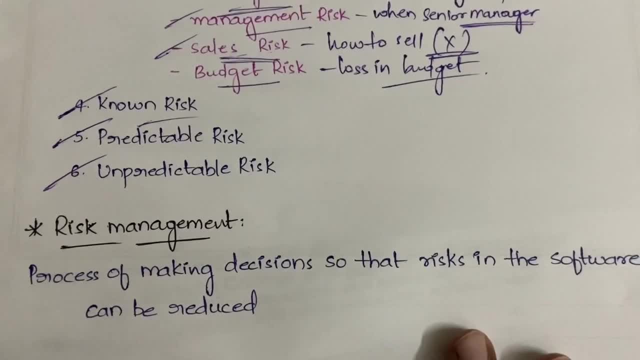 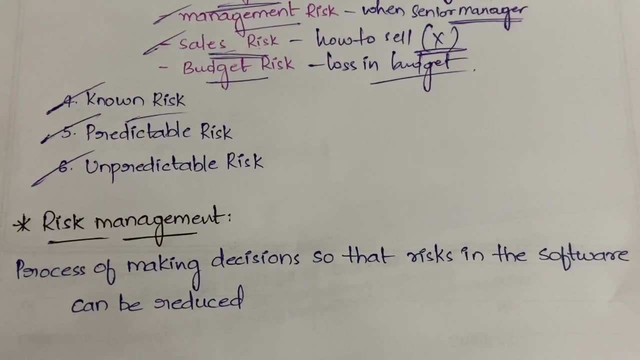 going to learn is- let me zoom in- so it is risk management. so what do you mean by risk management? as i said, i'll be explaining about risk management as well. right, so risk management is nothing, but it is a process of making decisions so that risks in the software can be simply managing the risks. 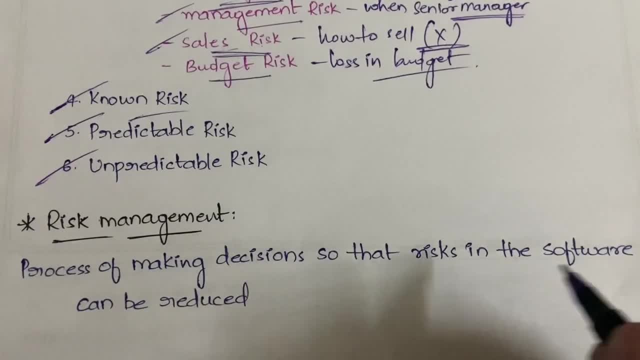 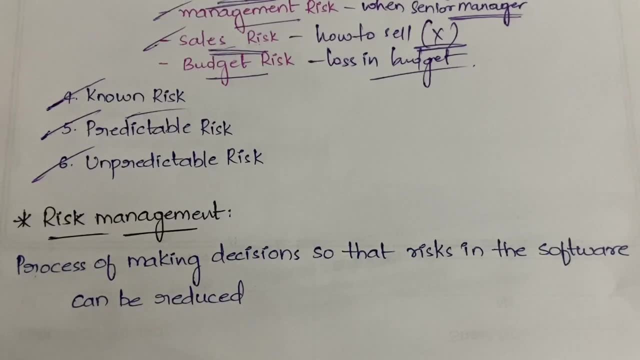 ready using the risks. okay, it is a process of making decisions so that the risks in the software can be reduced. or you can also say it is a process of reducing the risks in the software. it is a process where the risks in the software can be reduced anything your wish. you can add it on your own.